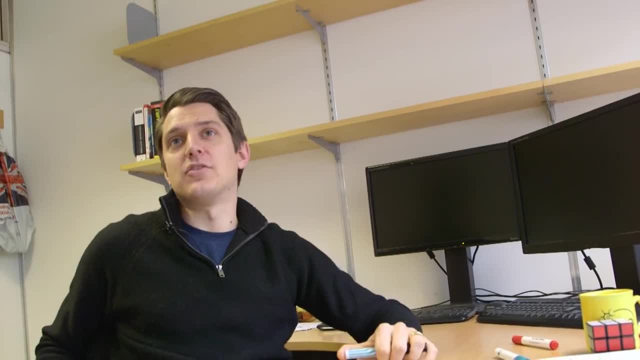 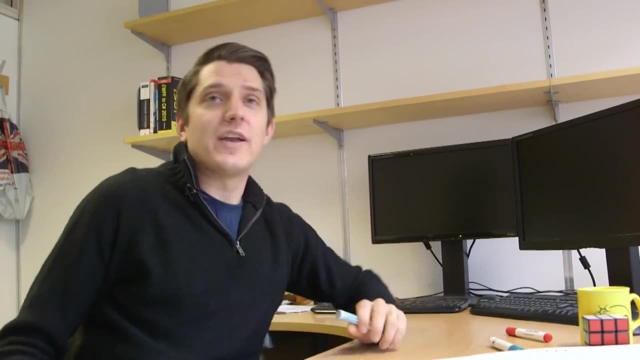 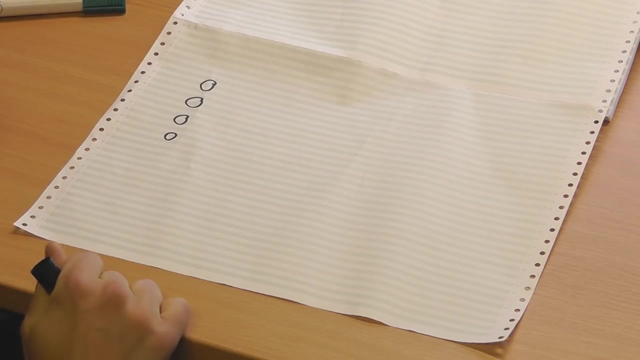 So that's the kernel convolutions we did on graphics and things like SoberLocker- Yeah, SoberLocker- Gaussian Blurs and things like this SoberLocker in particular- and Edge Detection. So if we think back to a traditional artificial neural network, what we've got is we've got some kind of input. we're trying to learn. 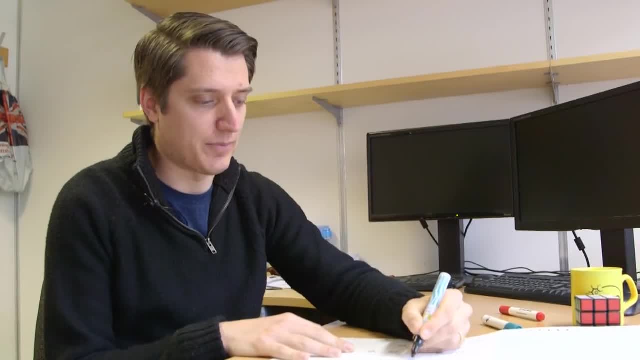 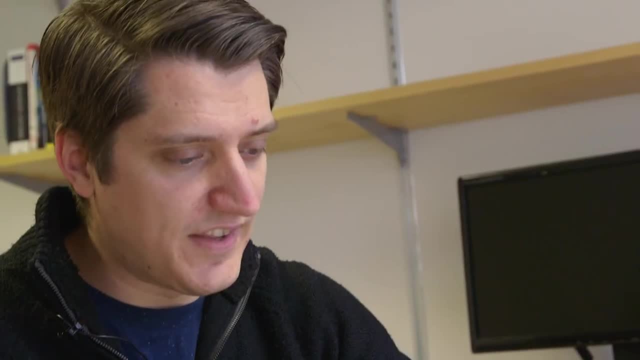 We've got some hidden layers and then we've got some output layers- Maybe there's just one, I don't know- And these are fully connected. so we have lots of connections from here and here and here, And then these are connected to here and so on. I'm just drawing in a few of them And then these are all connected to the end. 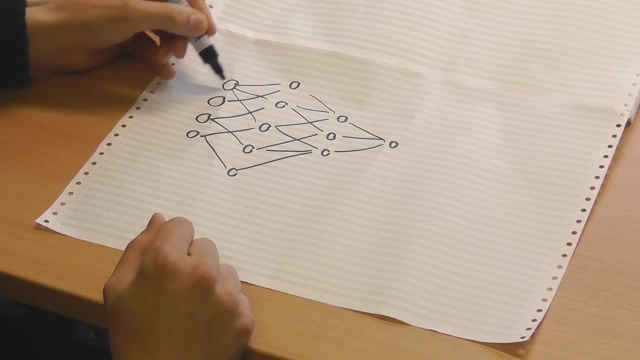 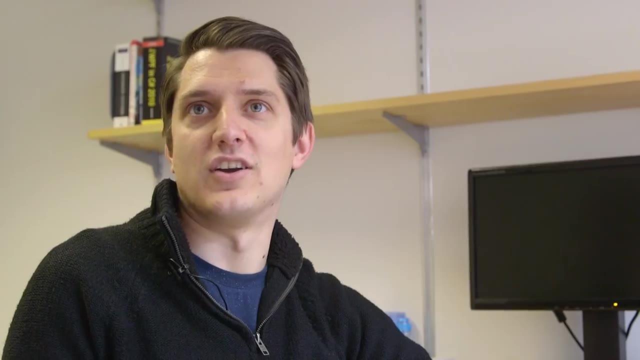 Now, using Bryce's analogy. we were talking about house prices, So this would be something like number of bedrooms. This would be something like: has it got a pool, And this would be you know what floor space is it, And has it got a good garden, And so on. 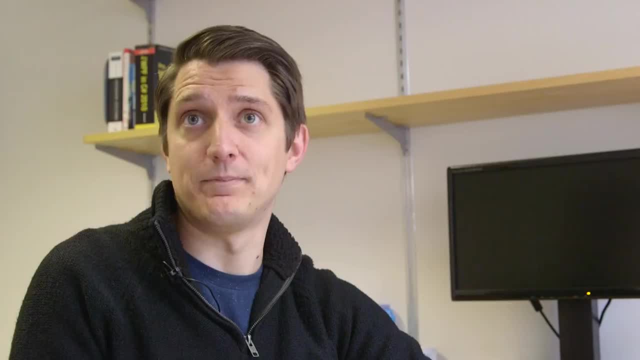 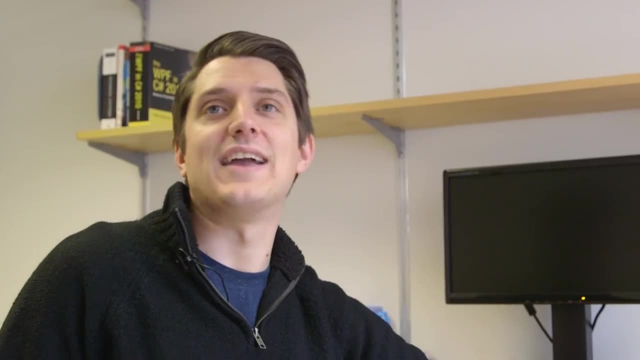 Lots of these, okay, Lots of inner nodes that we don't really care about particularly Well, I don't right, And so on and so forth, And then finally, at the end, we have a house price. Now, what this house price is is a complicated function of these inputs. 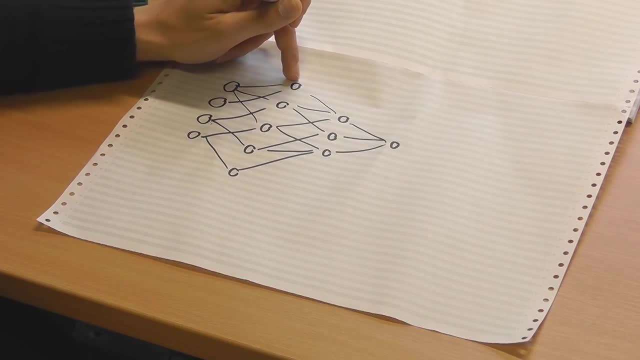 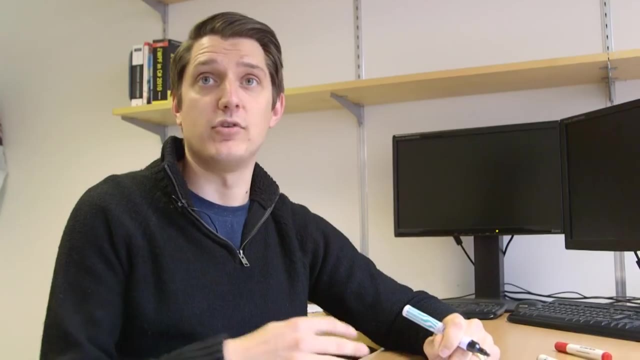 It's complicated because this node here is some linear or nonlinear, now combination of these. Okay. so a bit of this plus a bit of this, plus a bit of this plus a bit of this Through some nonlinear, Through some nonlinearity function. 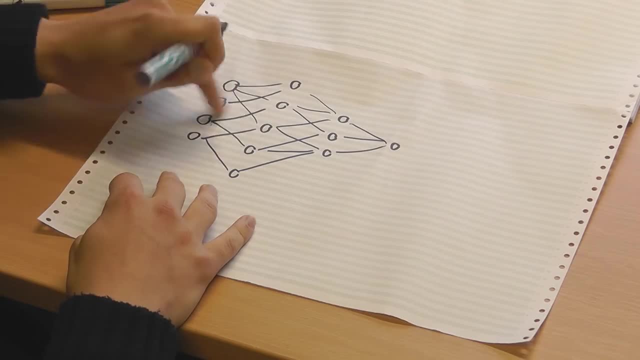 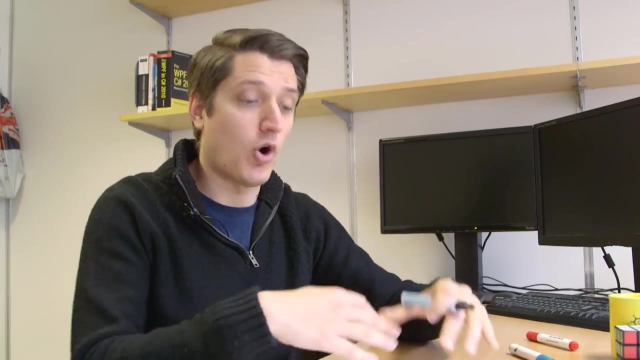 This is a different combination of these, This again different combination of these, and so on, right And then this is a different combination of these. So you can see, you're building up some kind of level of abstraction here where you've got combinations of combinations okay. 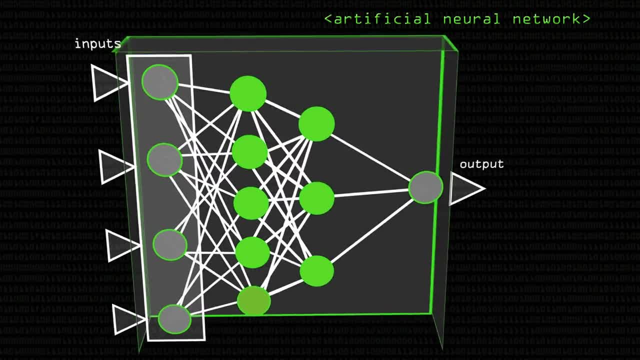 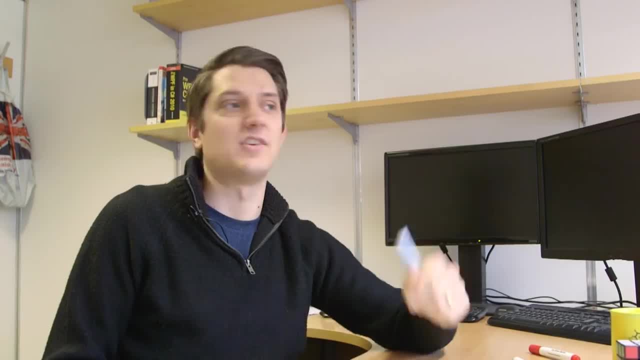 And that function is very complicated. When Bryce talked about a black box, in some ways that's exactly what it is, Because we can't look at these individual weights and say: well, that's got point two of this one. so that must mean this. 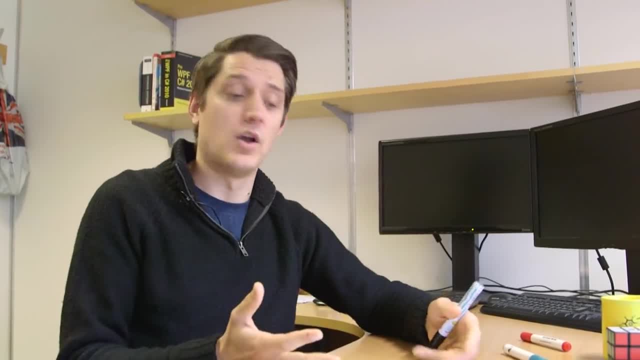 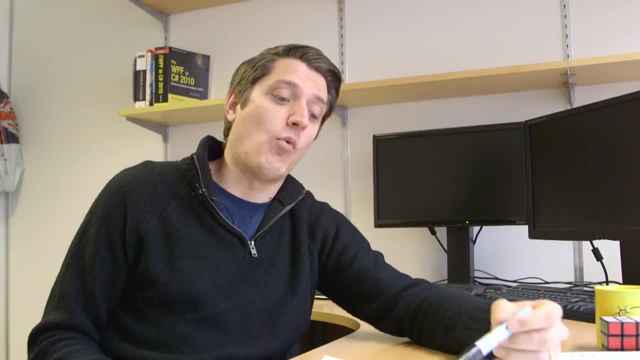 Because we just don't know what it means, right, In the grand scheme of things, in this whole network, we don't know what that individual weight means. Okay, and, to be honest, we might not even care that much. What we really care about is: how well does it predict house price? 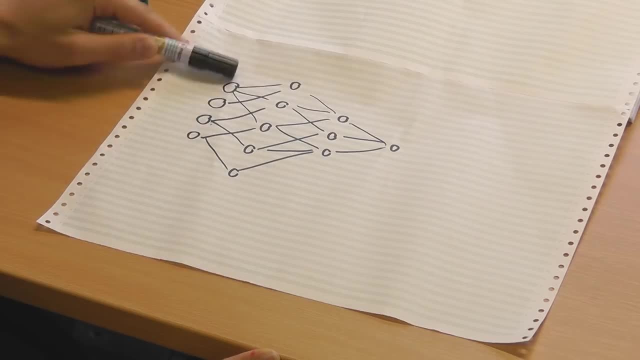 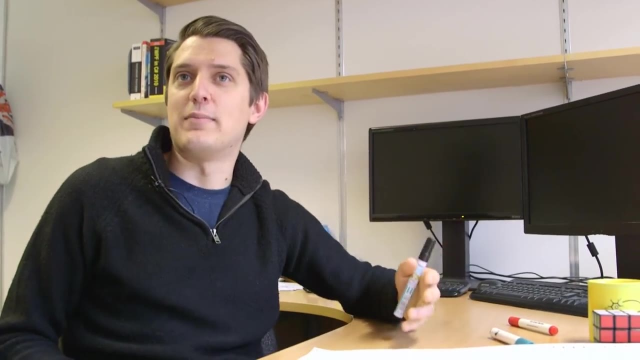 How accurate is that? based on that, for a different input, So we change this. read the output. is it good? Yes, brilliant. Okay, now for images, which is obviously what I spend most of my time around. this is a start, but it's not very useful to me. 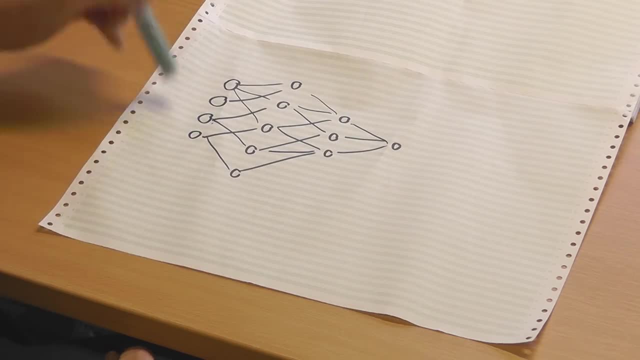 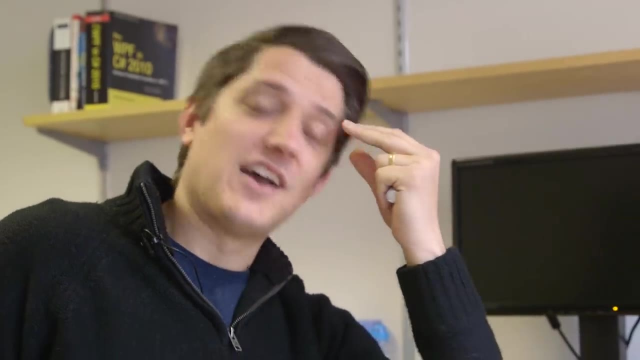 If you think that this is our input, okay, and I give you a picture of a house and I say: right, tell me how much this house is worth. Okay, well, what? So? how do I? okay, so there's two things I could do, right. 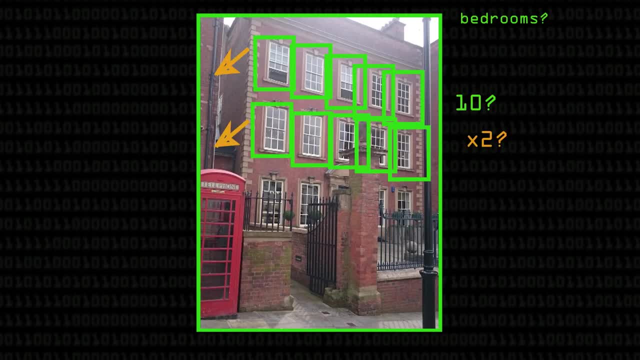 First of all, I could try and calculate things like number of bedrooms and stuff based on the image and put them in here. In some way I'd be calculating some features and then I'd be putting them in here and learning on those features. 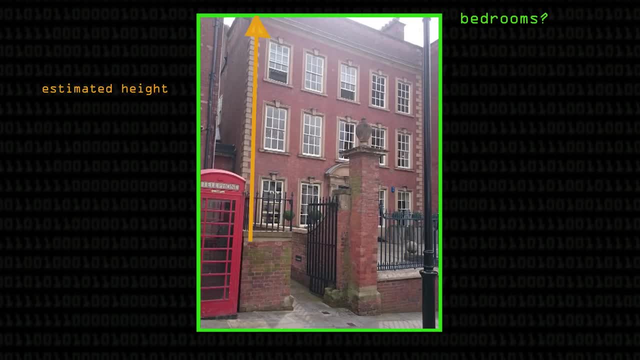 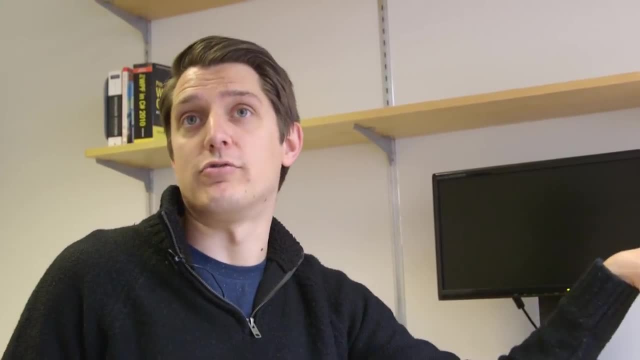 That is quite a smart way of doing it, because apart from that it's obviously quite difficult. It's smart because we don't have to have that many more neurons In anything. we can actually use the same network as we used before for our model on our house. 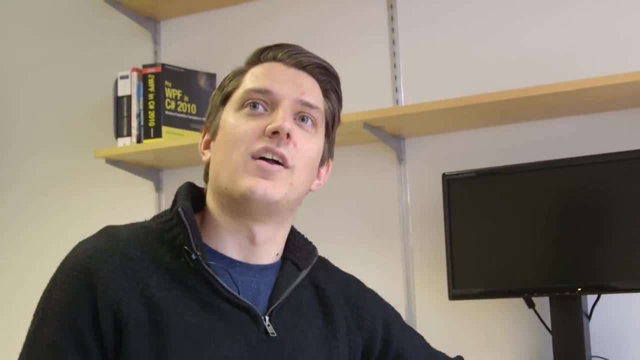 All we have to do is work out the bit of code that does the image analysis. Now anyone that's tried to find out the number of rooms in a house based only on one picture of the outside of the house will tell me that that can't be done, right. 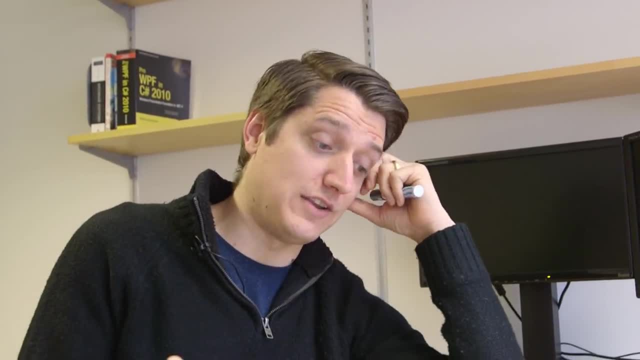 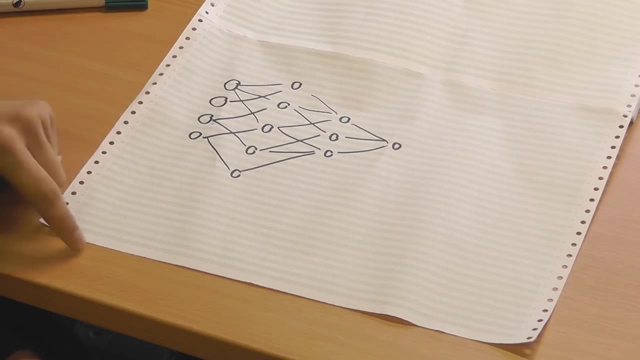 That's hard, okay, So you could naively think what we could do instead is just put the image in here, make this the first pixel and this the second pixel, and this is the third pixel, and so on. okay, Then this has got all the information it could ever need, right. 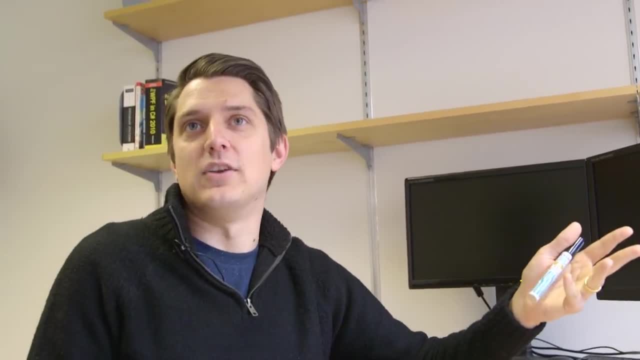 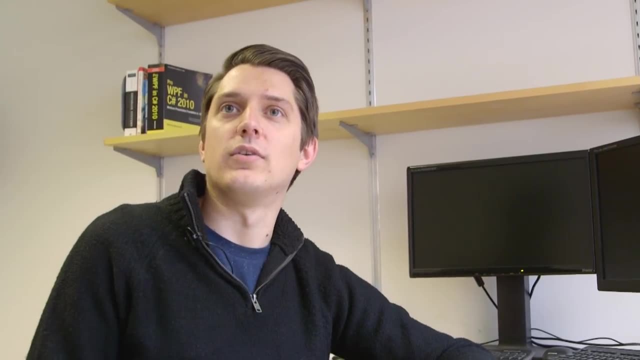 But that's the problem. okay, Seven megapixel image that's seven million input nodes. Let's say we have seven million nodes on the next layer. Each one connects to each other one. You can see that that's just going to melt my computer. 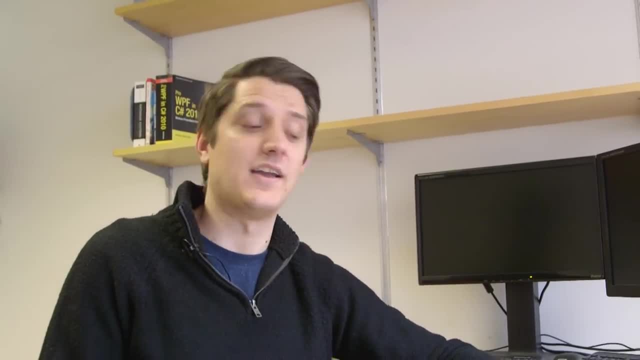 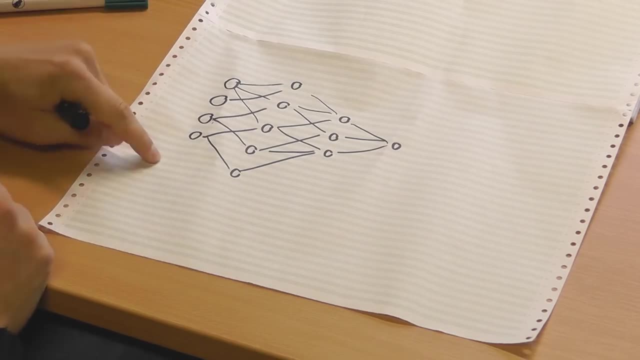 It's not even going to try and create it. It's too much information, okay. That's why we downsample our space a little bit. What we would usually do is calculate some small subset of features and then we would put them in at this end. 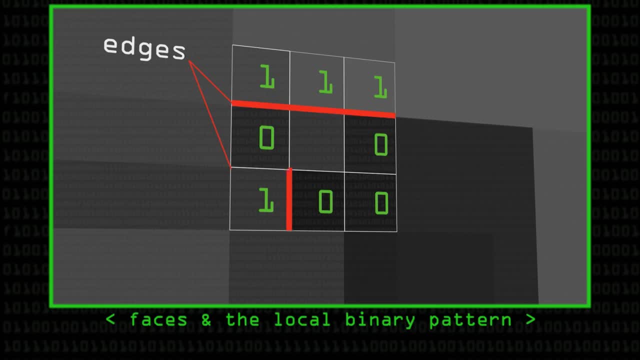 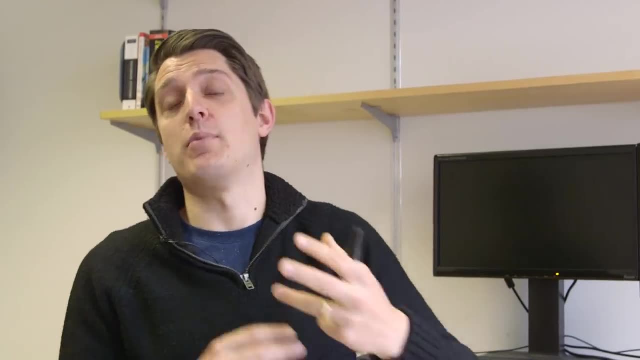 So that's quite important. So traditional machine learning is done a bit like that. So Michelle's done some videos on this: Calculate some features about someone's face and put that into some machine learning algorithm. What you don't do is try and put the machine learning algorithm. 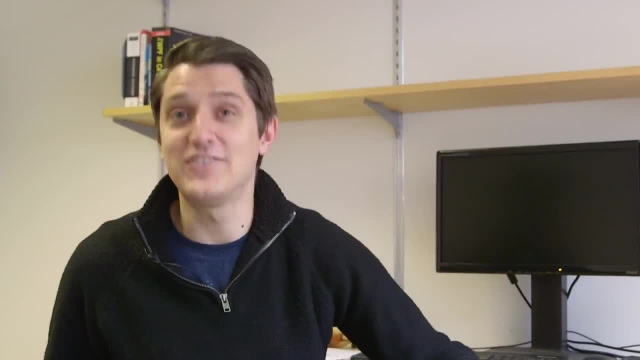 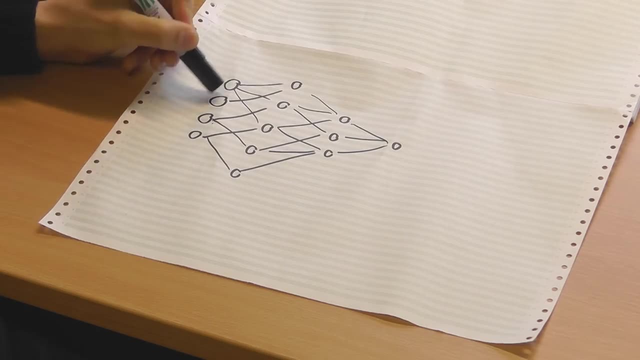 just on the face, because there's too much information there Until now. okay, That's where convolutional neural networks step in. So convolutional neural networks replace each of these nodes with a kernel convolution, so like a Sobel edge detector. 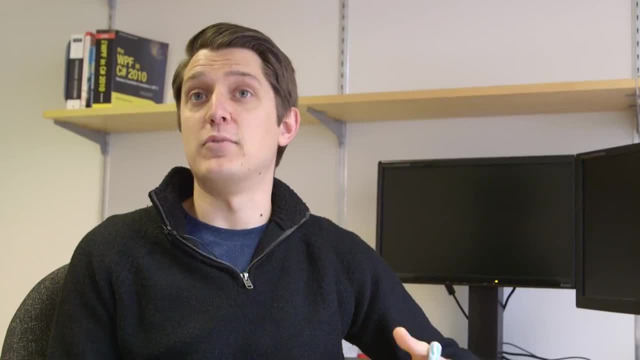 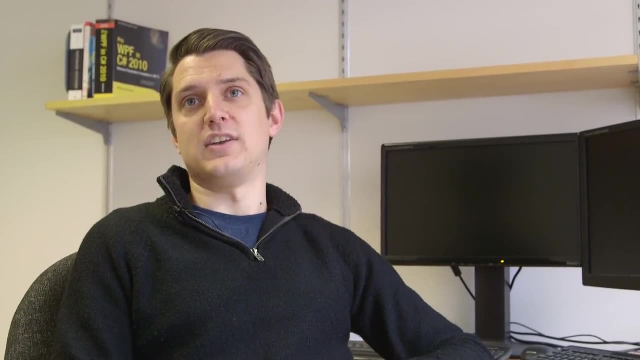 So instead of what I would have done before, which was run a Sobel over something and then machine learn on that, I just give this the opportunity to learn which features are interesting. Maybe it is an edge detection, Maybe it's a corner detection. 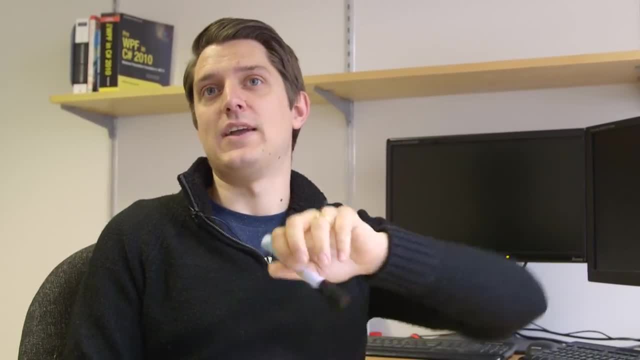 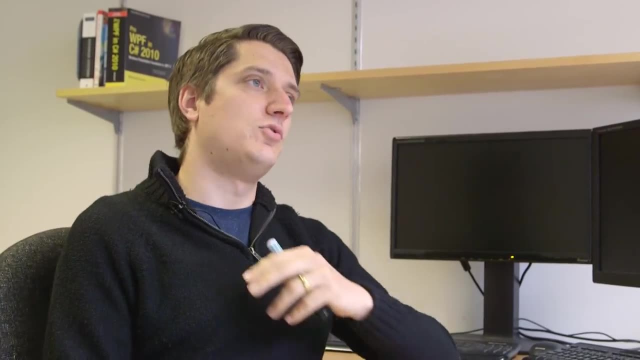 Maybe it's something that highlights whatever's in the middle of the picture, or something that highlights the top left-hand corner. It doesn't really matter. and the point is I don't know what they are. If I give you 2,000 pictures of houses and ask you to predict house price based on the 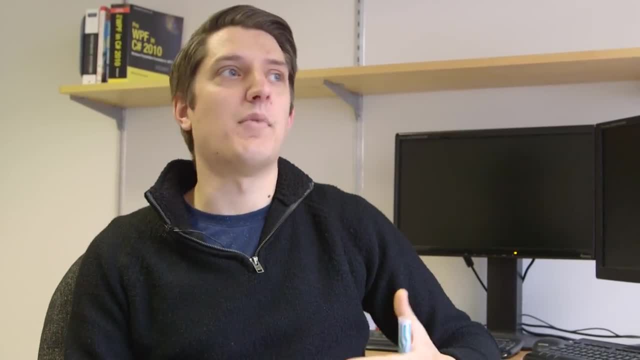 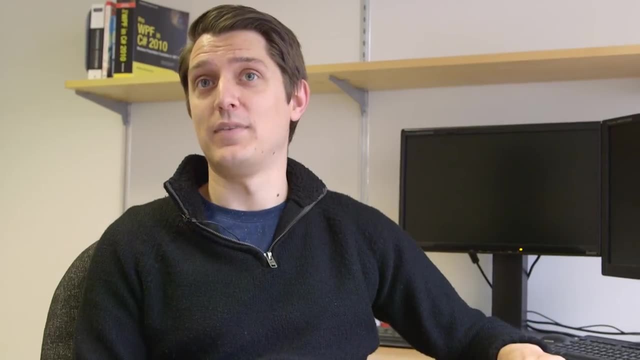 pictures. I don't know for sure. I can guess that it might be how many windows it has and things like this, but I don't know for sure. A computer can brute force through those things much quicker than I can and tell me and then 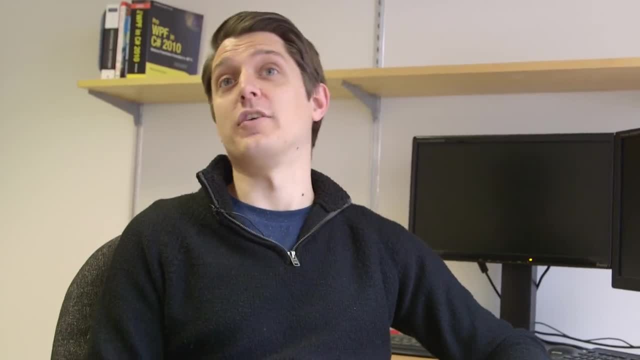 I can go, I can both predict it and I can look back and say: oh, it was windows after all. So let's imagine that what we have is our image. So I'm going to move away from the house analogy now because I'm going to have to draw a lot. 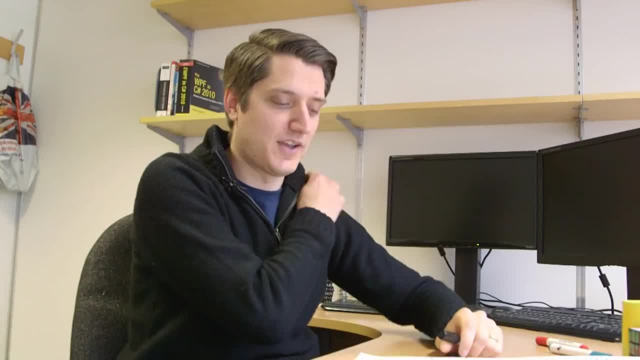 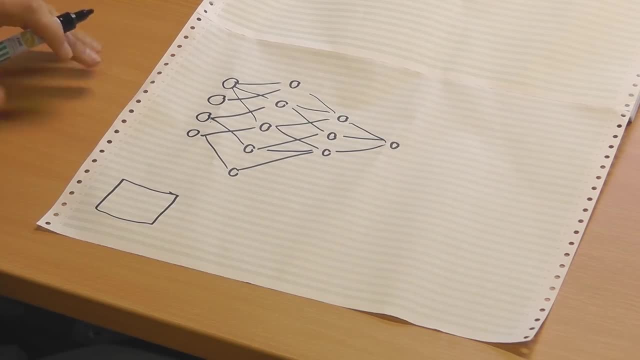 of pictures of houses if I do that. So let's talk about how CNN works and why it's useful. So we have an image of something Now. I have seen convolutional neural networks used for non-images, but for now we'll just talk about images. 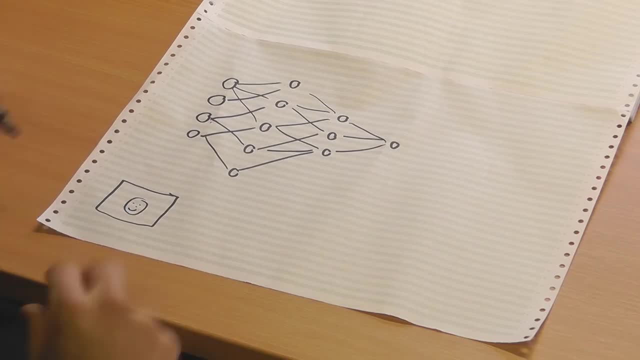 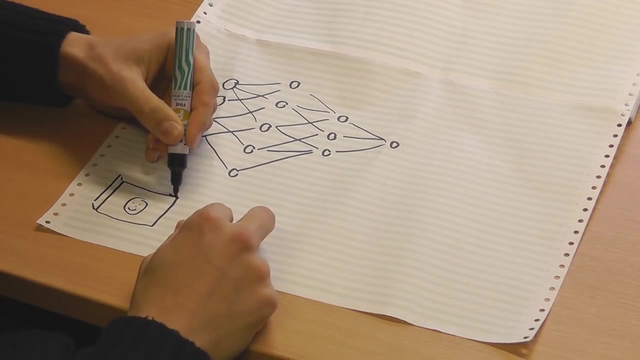 This is a picture of, let's say, me. It's not a great likeness, but I'll stick by it. Now, there are three channels here, So this is actually a 3D volume in some sense. Remember, If you had 3D images, you could view RGB as, in some sense, 3D. 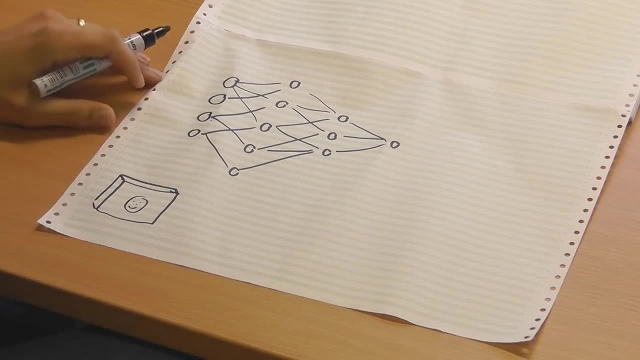 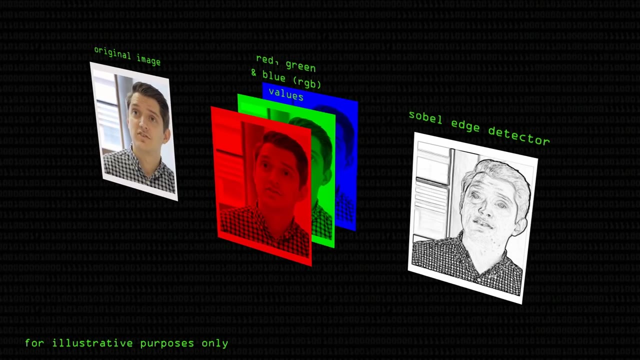 So the first plane is R, G and B or vice versa. What we do is, if we performed a Sobel edge detection on this, what it would do is produce another image that was slightly smaller than this and only one deep. So hypothetically it would be another image where the edges, let's say the horizontal, 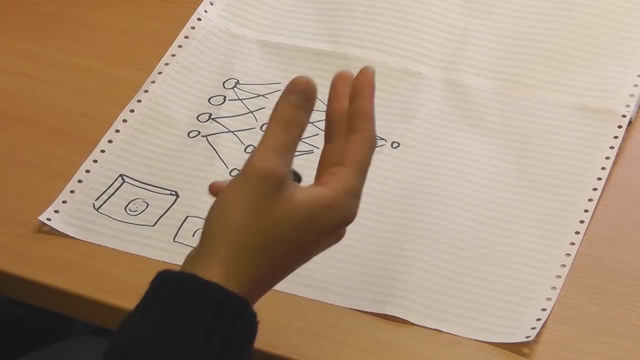 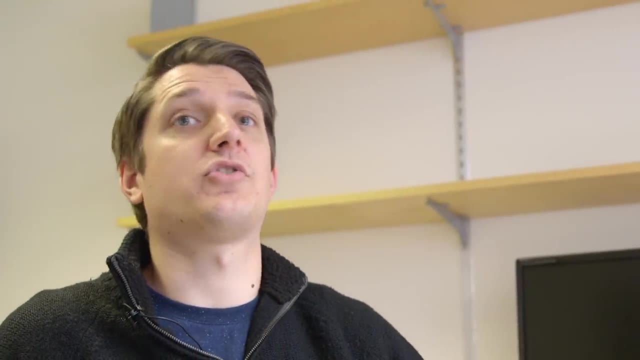 edges were highlighted. So it would kind of look like that or something, I don't know: some half of my face where the horizontal edges are highlighted. It's not a great diagram, but there would only be one output because Sobel just outputs. 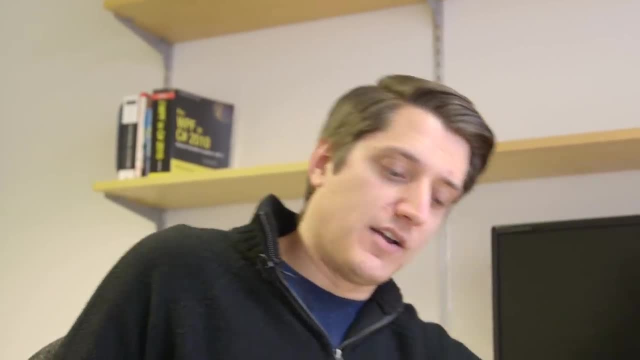 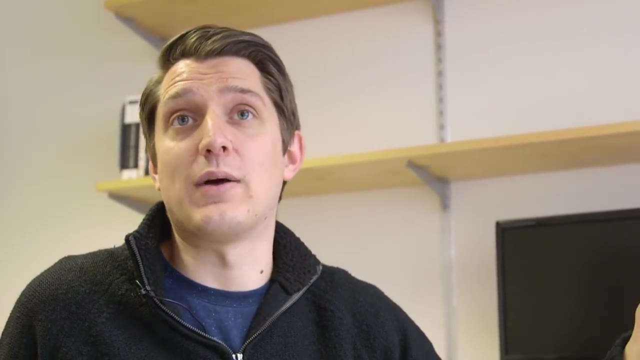 a number between 0 and 255 as soon as you scale it. Now the problem is that I don't know that Sobel's the best thing for this task. It might be. It might be useful to detect edges on houses, to work out what the price are, or if you 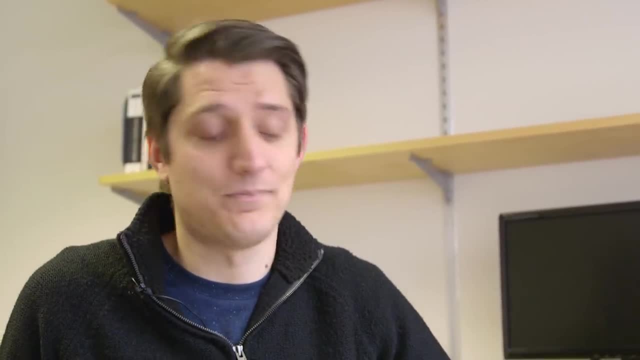 want to detect faces, to detect the sides of the faces. That kind of makes sense. On the other hand, it's going to produce a lot of erroneous bits. If I'm sitting in front of a tree, there's going to be loads of edge stuff going on there. 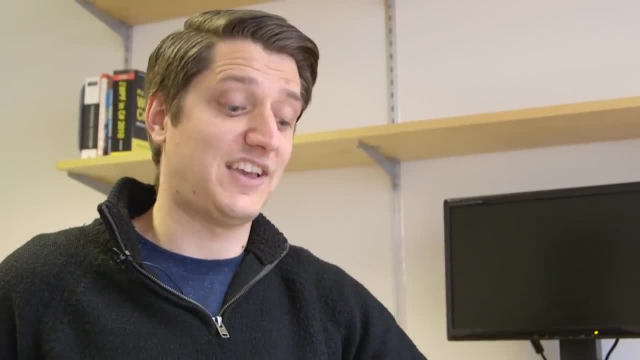 that I don't care about. In a convolutional neural network, what we do is we do, let's say, 60 of these on the first layer, So we have one, and then behind it we have another one, And behind it we have another one. 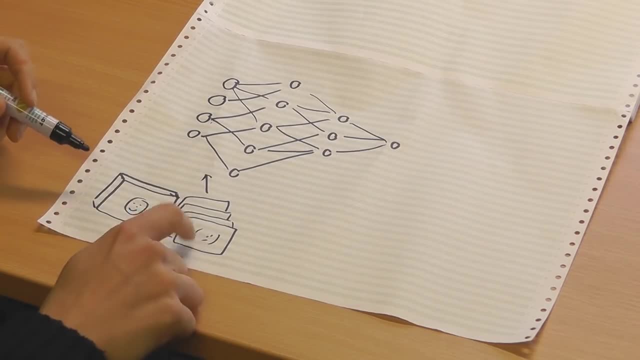 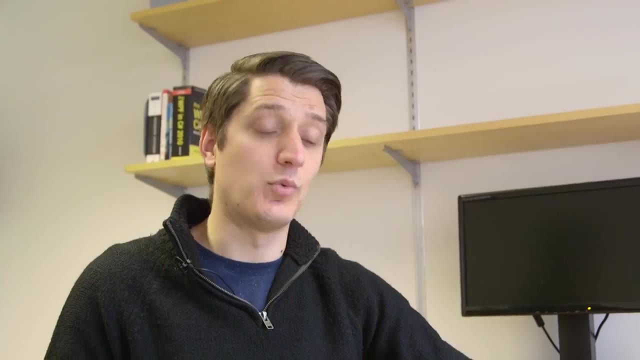 Behind it we have another one, And so on going this way. So the first one will be some convolution process applied to this whole image that takes three input channels and outputs one output channel. The next one will be a different kernel convolution operation. 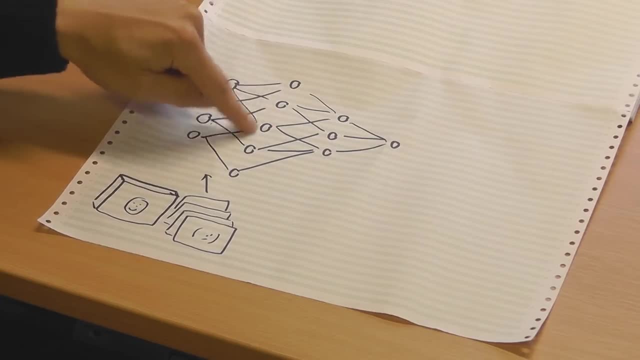 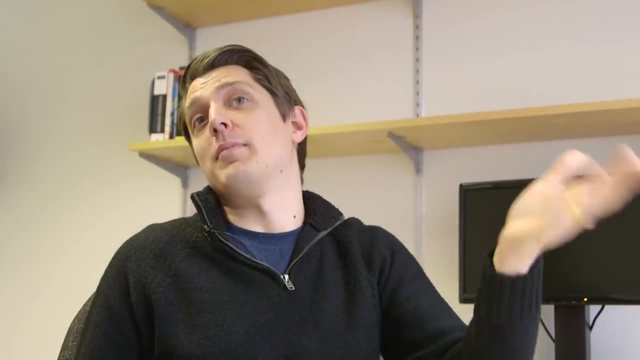 So each of these will have a different kernel. Those are our weights. Those are these values here instead of our analogy back to normal learning. And so let's say we have 60 of those or 64 of those. One of them might be detecting edges. 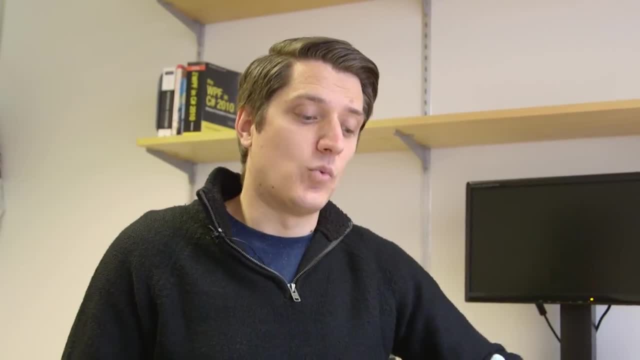 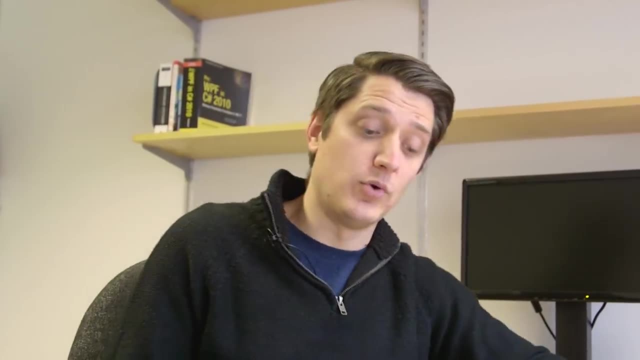 One of them might be detecting corners, And then we use that. We use them as our features for learning. Now, that's a start, but this is deep learning now, right? So what do we do now? Well, what we now do is we do more features based on these features. 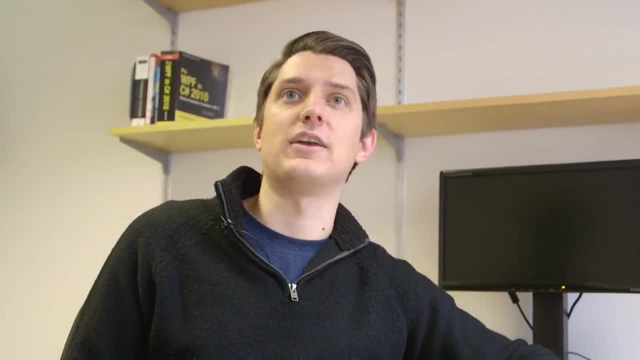 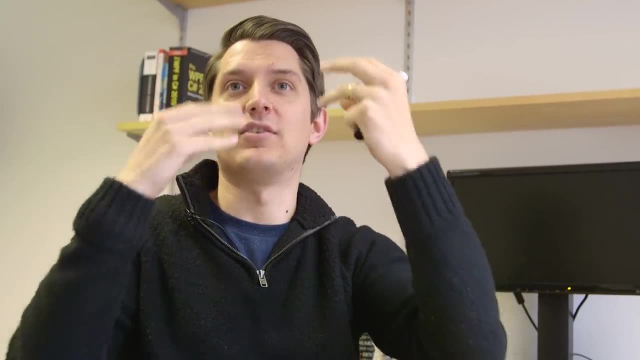 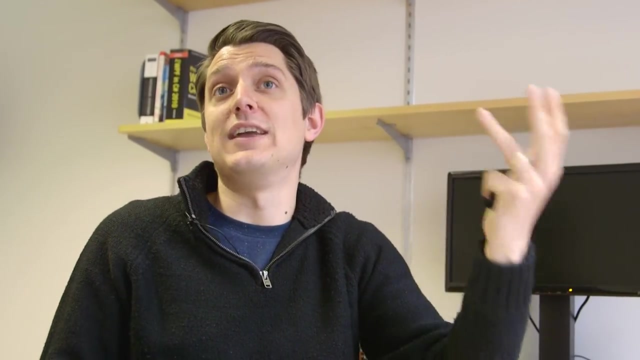 So we find combinations of corners, combinations of edges that make something interesting. My face is not just a circle of edges. What it is is a number of corners and edges and bits of texture and things, all in a specific shape that is unique to- well, certainly to a human face, but even unique to me, right. 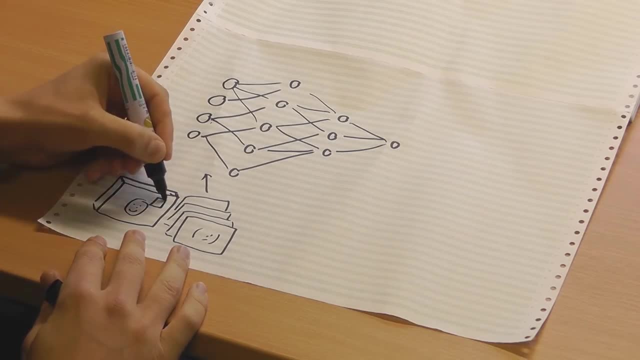 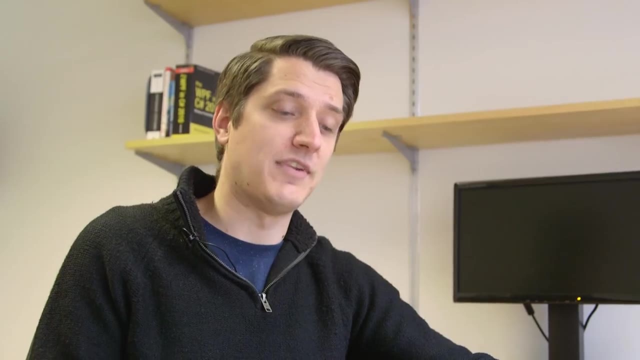 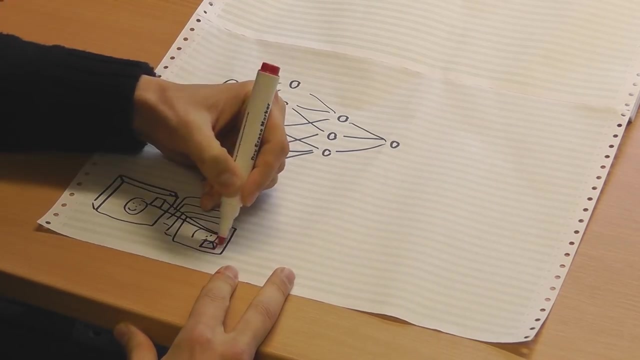 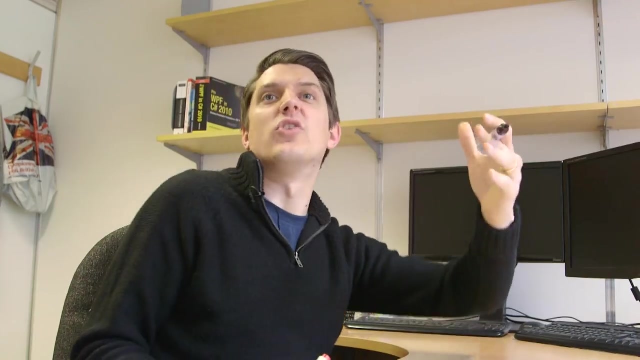 These are capable of distinguishing between different shapes. All right, So what we would like to see now is how many corners we have. Okay, now, we have just layed these together here. Now. what we'd like to do next is take a little more of the. 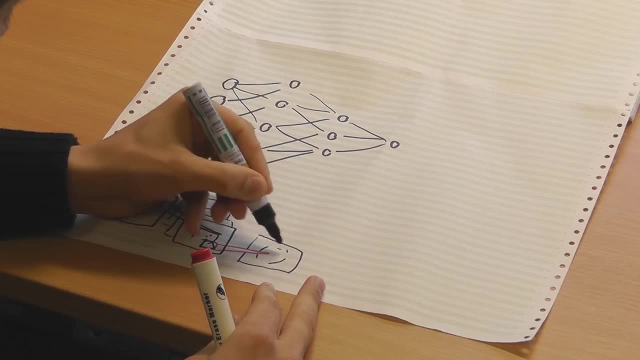 color, Our color goes in White. We're going to use some contrasts. It's not going to make much sense to us, but it'll make some sense to this machine And there'll be another set of these, so there'll be lots of these going back. 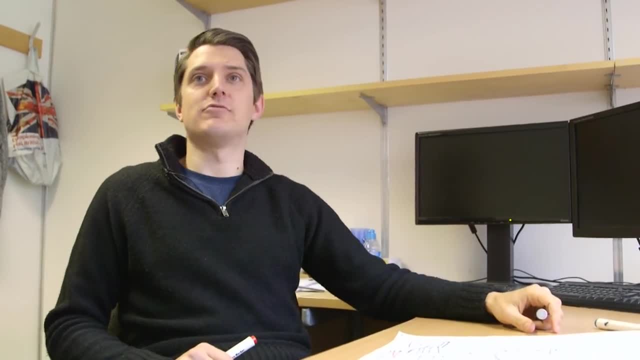 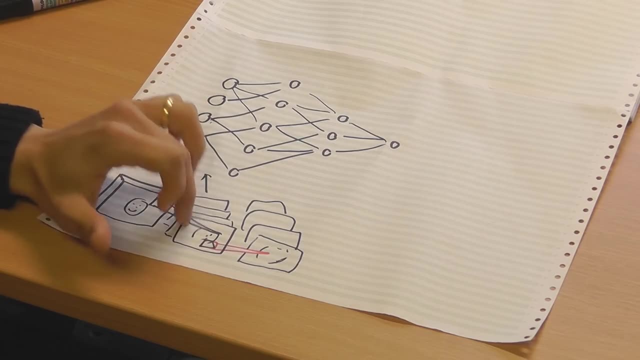 All of these will look different and be some different representation of my face transformed in some way to be useful. And again, I haven't picked these. These have been learned just like a normal deep learning algorithm. So I haven't had to say I definitely think edges are important for this, because I don't know for sure. 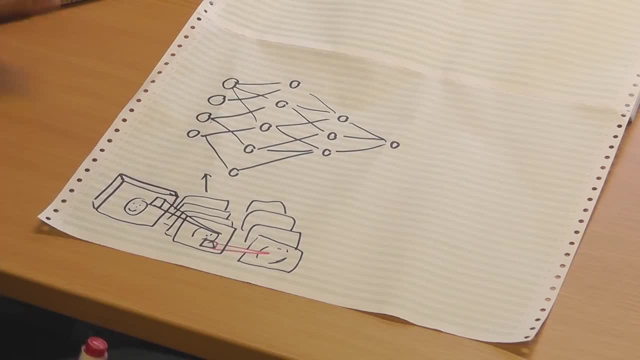 So this goes on and we keep doing this, And sometimes we also downsample the size of these images just to save memory, But we won't dwell on that too much. And because of the way that we downsample and the way that sometimes these convolution operations slightly shrink the image, 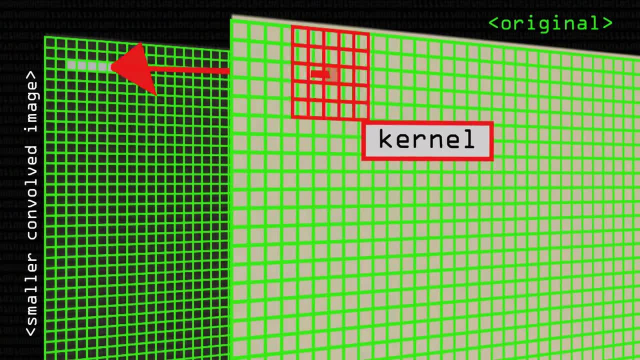 because they don't go all the way to the edge, right? If you've got a 5x5 kernel, you can't go to the edge 2 pixels because you're going off the edge. So we don't worry about that, We just get slightly smaller. 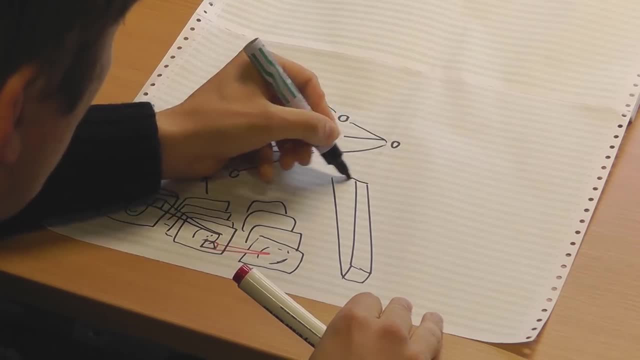 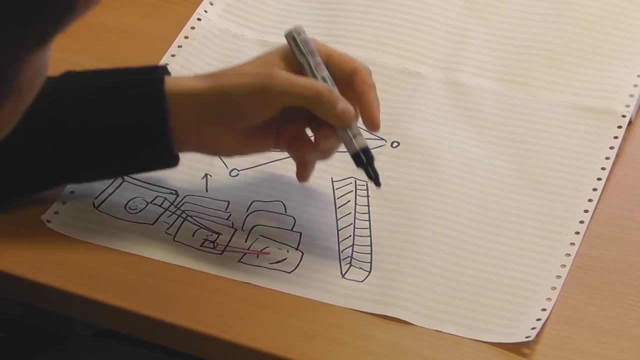 In the end, we end up with a much smaller image and lots of features going all the way back. So these are my different convolutions of convolutions, of convolutions of convolutions, And each one will look different and represent something different, And we don't know what they are. 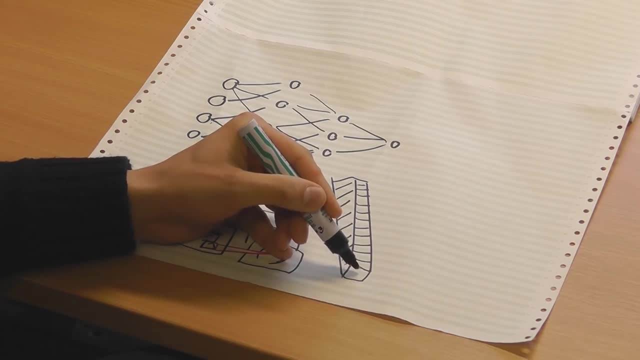 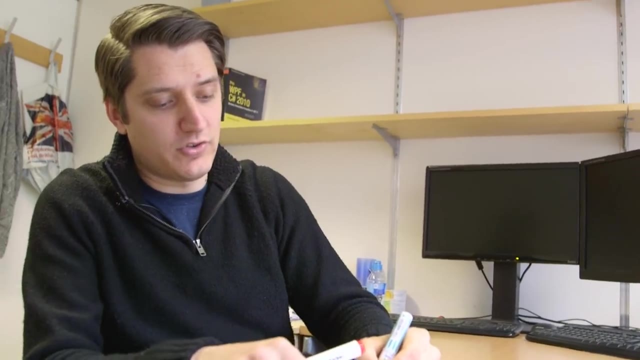 So this one could be highlighted when there's a face in the middle, or it could be dark when there isn't. This one might be highlighted when there's an ear at a certain position, and so on. Eventually, these will get down to being just one pixel and very, very long. 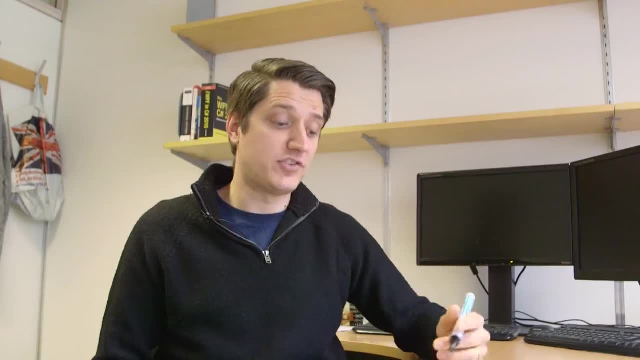 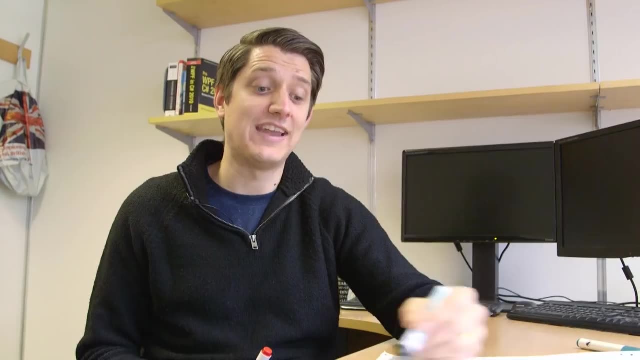 So essentially, what we've done there is: we've completely removed the spatial dimension. There's no more spatial information left. We don't know where anything is, but we know what it is because it's listed in all these features. These now are our neurons at the end. 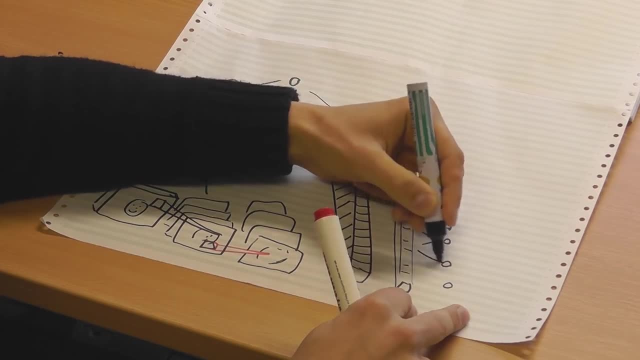 So we have a couple more layers that point to these, And then, finally, we have one at the end that says: is this a picture of Mike's face? And it produces a one if it is and a zero if it isn't. 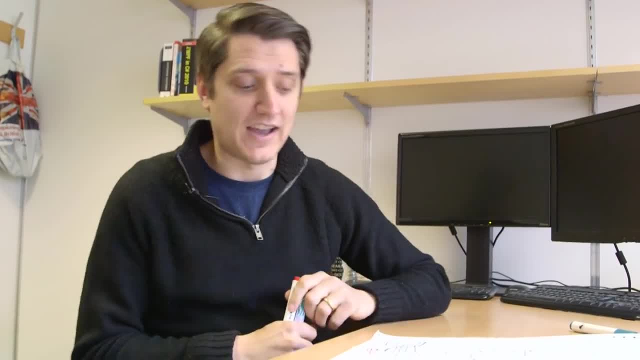 And then what we do is, just like a normal network, we train it. So we say here's a picture of me, So this should be a one, And let's say it's a 0.5, because it's kind of random. 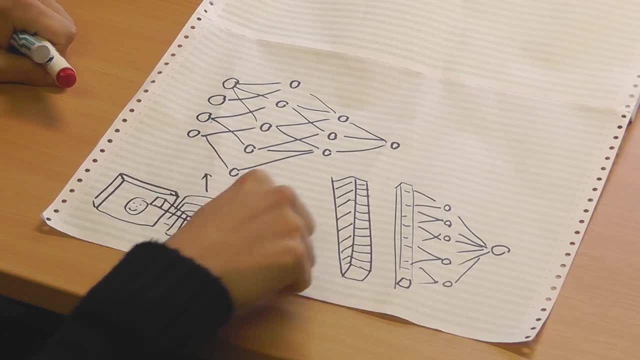 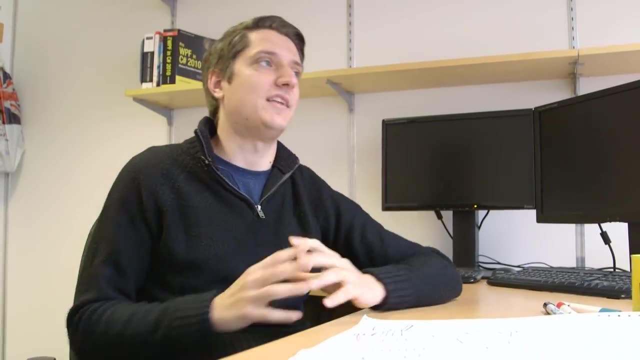 So we adjust these weights and we adjust the weights inside all these kernel convolutions. So does that adjustment happen manually? No, it happens using a Well, it's coded in, but it's usually performed by a library And it's using a process called backpropagation. 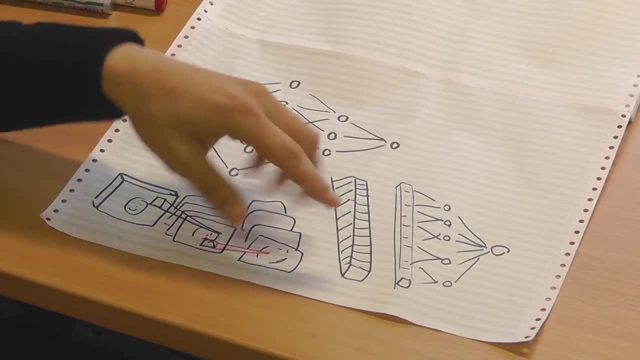 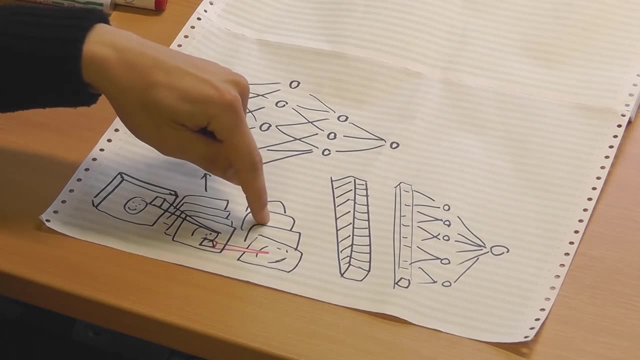 So what we do is we basically predict what direction we have to move the weights in to improve our output, And then we move them over slightly in that direction, And we have to do it in reverse order, Because these ones depend on these ones depend on these ones, and vice versa. 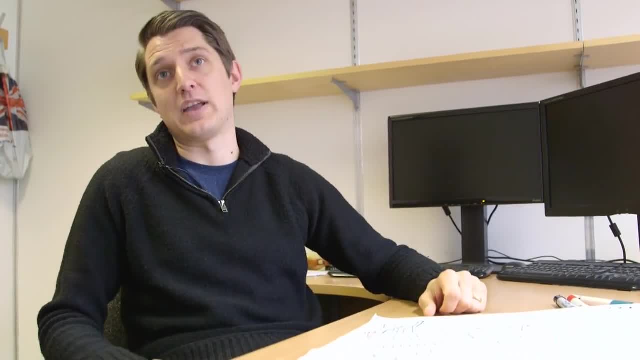 what we do is we say: well, look, given that I've said it's 0.5% chance of Mike and we want a one, how do I change these weights here to get slightly closer to one? And I do it. 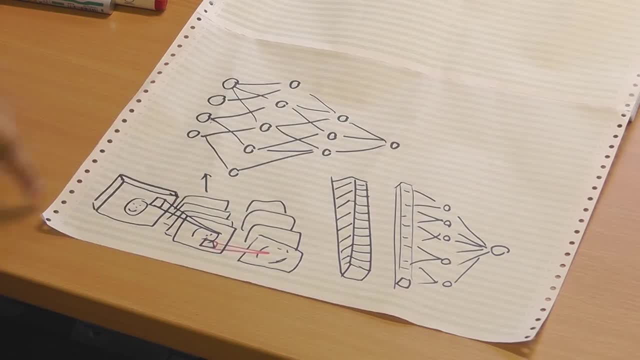 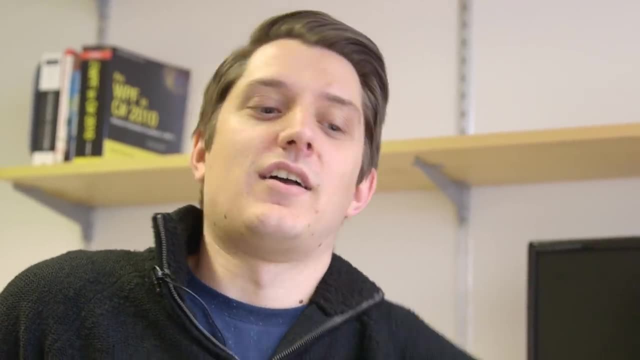 And then I say how do I change these again to do even better, And so on, and I work my way back. That kind of math we're not going to go into. A lot of these things are implemented in libraries. So as a researcher, I mean much as I'd like to implement some of these things. 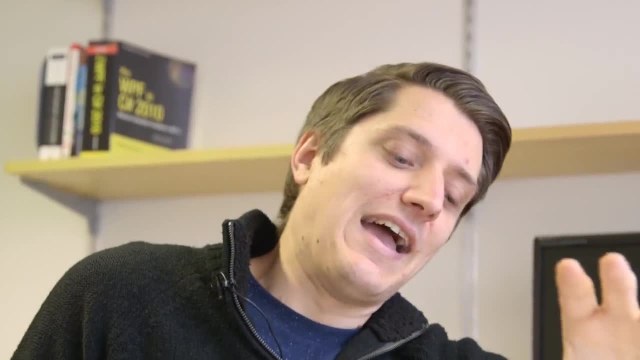 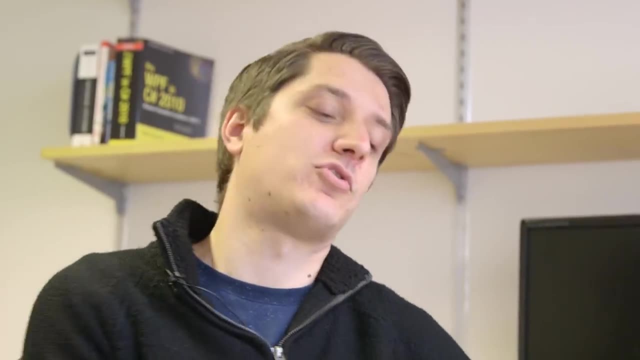 it takes quite a long time just because programming takes a while, And it's better for me just to apply these things and get good results than it is for me to reinvent the wheel all the time, constantly. If everyone was programming the same things over and over again, no one would get anything done. 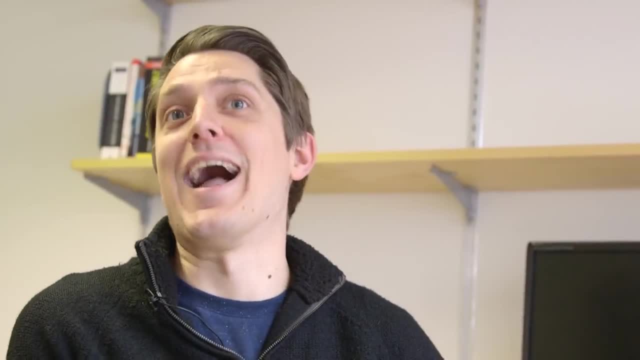 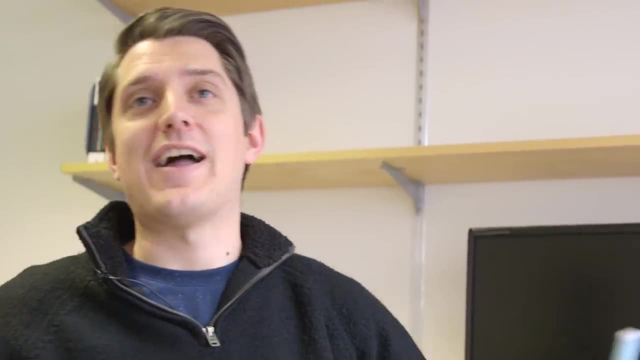 Because I'd have to start by programming up Linux to get- I'm not claiming I can, by the way- and so on. So let's not reinvent the wheel. So I do this: I send them, let's say, 1,000 pictures, 500 of which are me. 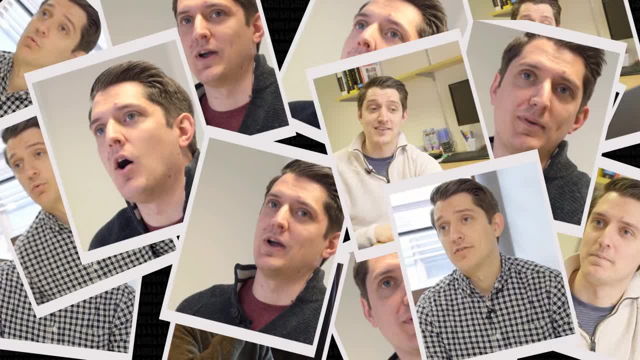 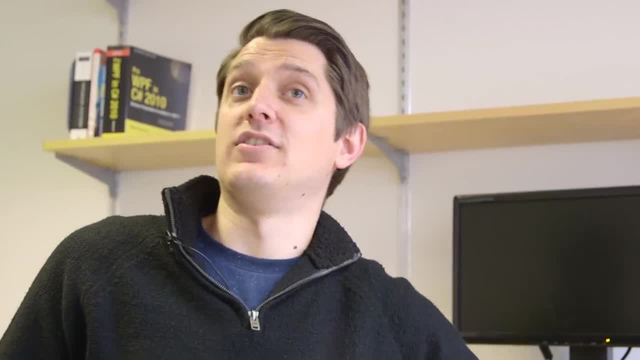 so I've been to a photo shoot or something like that, and 500 of which are not, And I train it. so the convolutions and these weights on the output are such that it gets one when there's a picture of me and nought when it isn't. 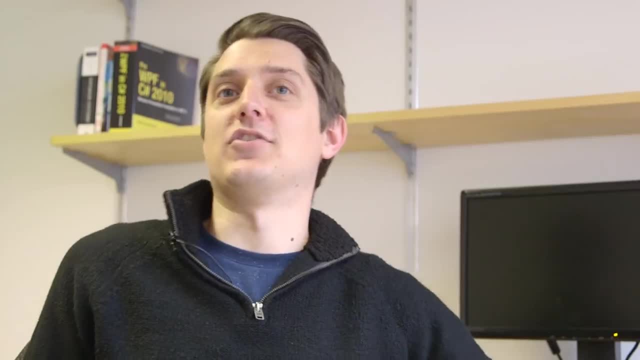 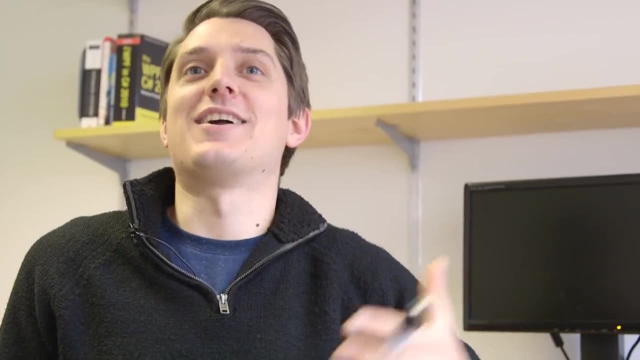 And then I can look at these convolutions and say: what is it about me that's distinctive, And it's probably going to be finding weird shapes on my face because it's a bit of a weird shape. So things that are unique to me. 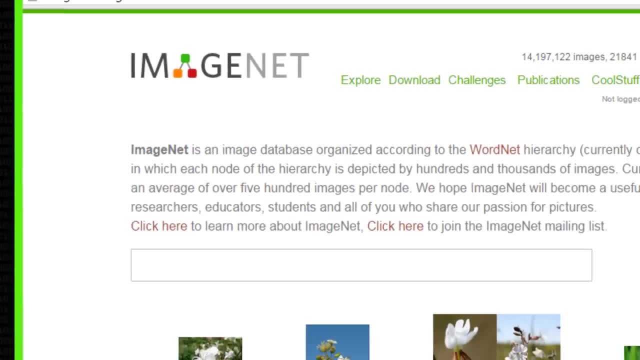 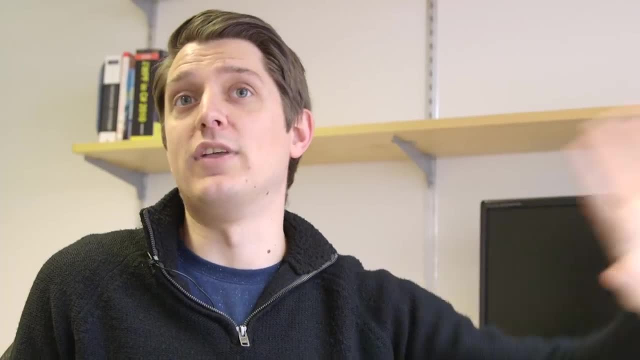 Now, in a more general situation, there's a big database called ImageNet. They have a competition every year to see who can classify these images the best. So dogs, cats, planes, trees and so on, They're all in there, and there's 1,000 or so images of each. 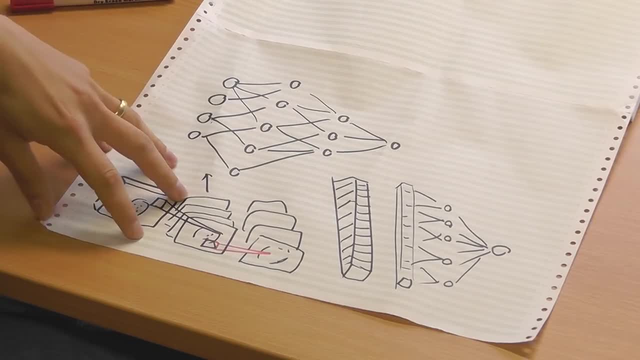 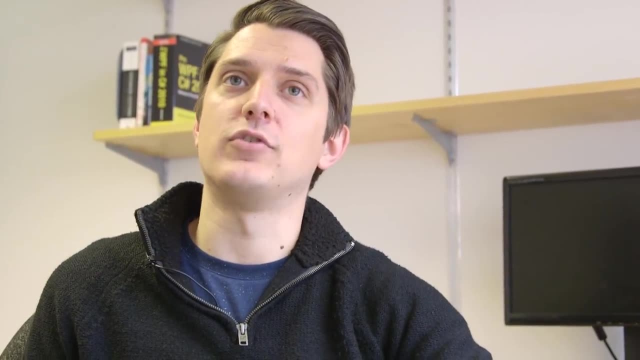 So we have a really big network, but it's much bigger than this little one I drew. and we say, right, let's throw millions of images at this, Thousands of cats, thousands of dogs, and we have lots more outputs than just the one. 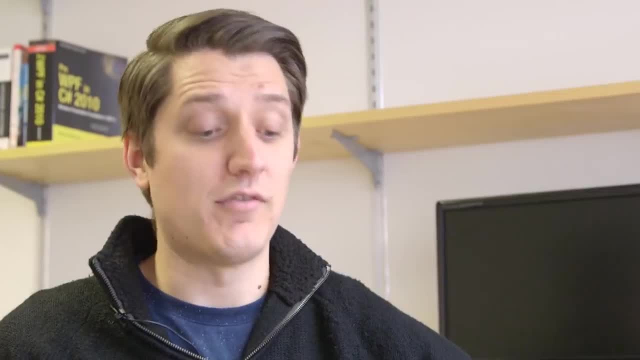 And we say what is it? And it says it's a dog And it is Convolutional. neural networks have been around for a little while, but they've really started to be big in about 2012,. when someone came along, applied one of these to ImageNet. 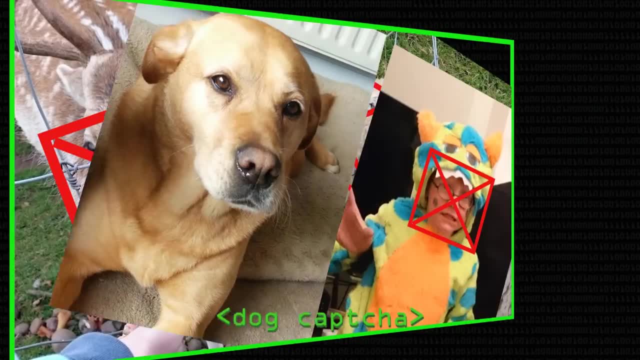 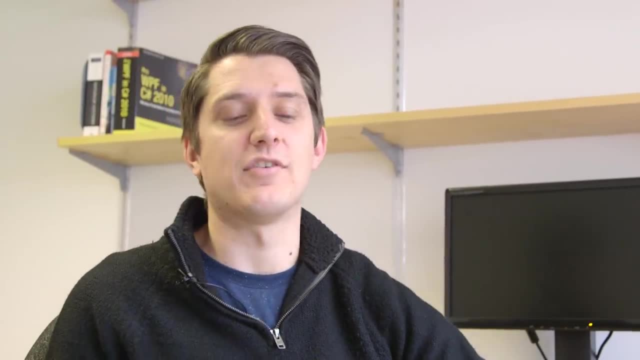 and got incredible results and so on and so forth. And now there's this big push and everyone's trying to get even better results and even better results. Now I work on more of the applied end of computer science, so I'm more interested in how this affects plant science and things like this. 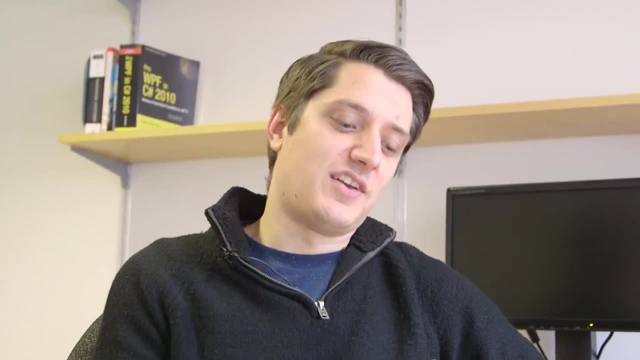 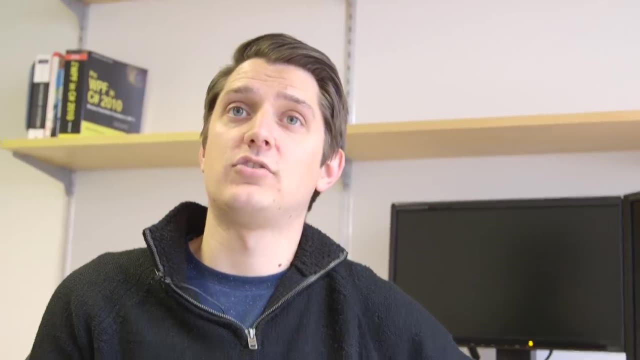 So that's what we're working on, But the kind of results we're seeing are really, really impressive. So I mean, case in point, I've done some root tip detection, so detection of root tips in images, Right, And I've got some software that I've already programmed.